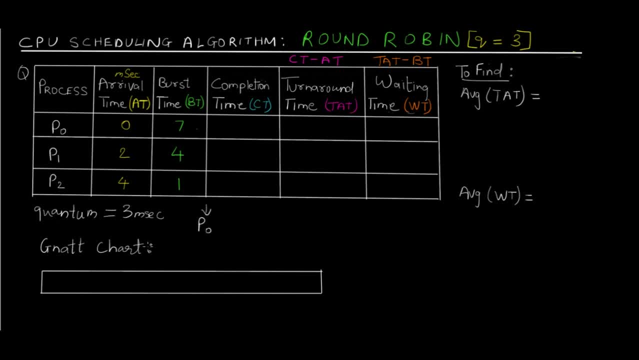 we know that P0 came into the queue, So let me just write down P0 over here in the Gantt chart. So this is at time 0 and we know that at 0th second there is no other process. So CPU will start processing P0 and 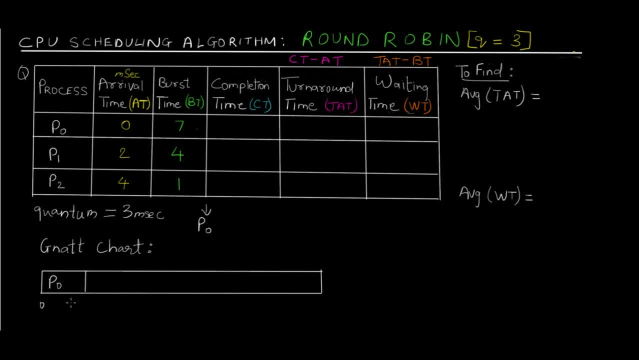 after 3 milliseconds, that is, after the quantum of 3 milliseconds, the CPU will see if there is another process inside the queue. Now we know that when 3 seconds have passed, P1 has already arrived in the queue, because P1 came in at time equal to 2.. So P1 has arrived inside. 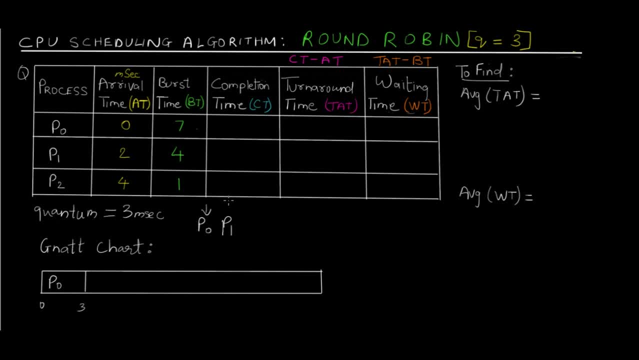 the queue. So now the CPU will stop processing P0 and move to P1, and P0 will again be added inside the queue. So you can see that CPU processed P0 from 0 to 3, but P0 actually requires 7 milliseconds. 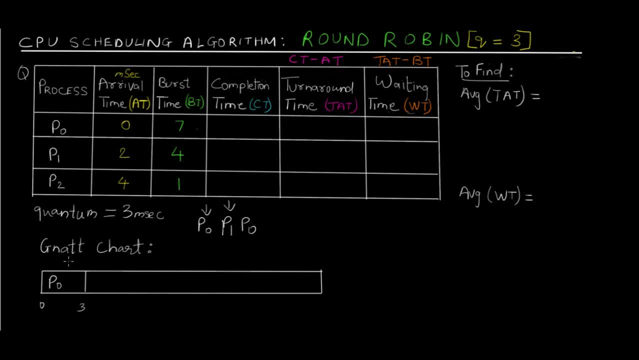 but CPU has only processed it for 3 milliseconds, So 7 minus 3, which we can write down over here, which is 4.. Now this 4 milliseconds is the time that the process P0 still requires to complete itself, But since the CPU has paused P0 and moved on to P1, from the third 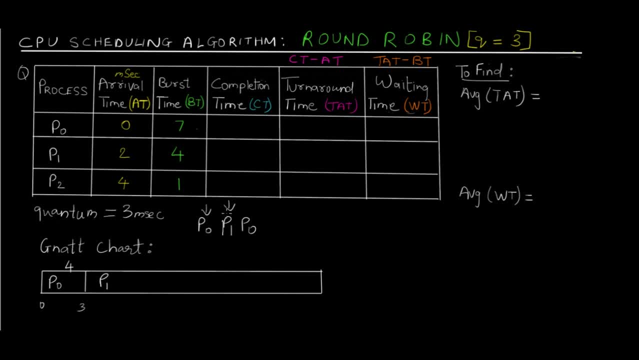 millisecond, we will start processing of P1.. Now the CPU is at P1 and P1, you can see, requires 4 milliseconds. So the CPU will first process it for 3 milliseconds according to the quantum. So that is 3 plus 3.. 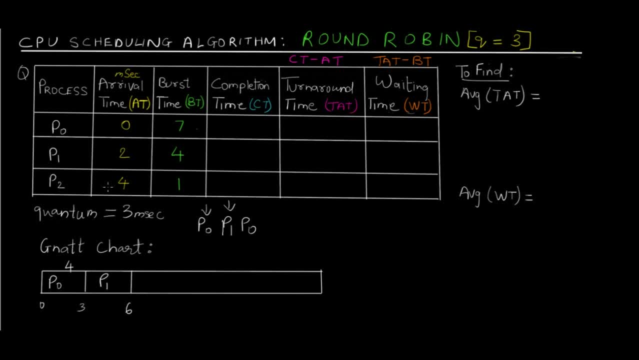 Which would give us 6, and by the time it is 6 milliseconds. we know that P2 has also arrived, because P2 arrived at 4 milliseconds. So you can write P2 over here and now. since the quantum is done, that is, P1 is processed for 3 milliseconds. Now the CPU will switch to P0, which is next. 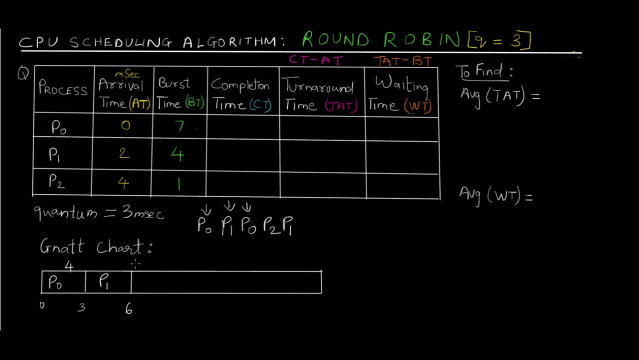 in the queue and pause P1.. So P1 will be paused and again added in the queue, because P1 required 4 milliseconds but it only got 3 milliseconds. So you can write down 1 over here and 1 millisecond is the time which P1 still requires to complete itself. So that is why we paused P1 and P0. 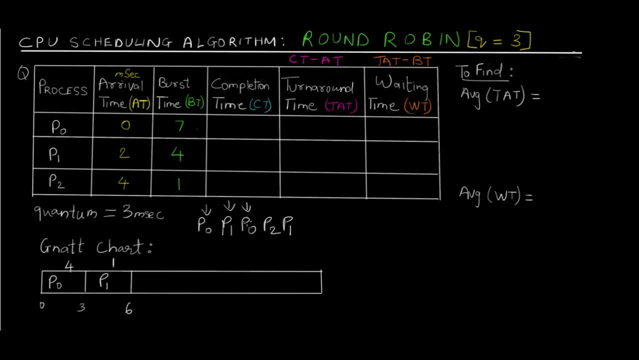 and added it inside the queue. and now we are on P0 again, because it was added inside the queue for the first time when it was paused over here. So now we know P0 requires 4 milliseconds. So let me just write down P0 over here. CPU will again process P0 for 3 milliseconds. that 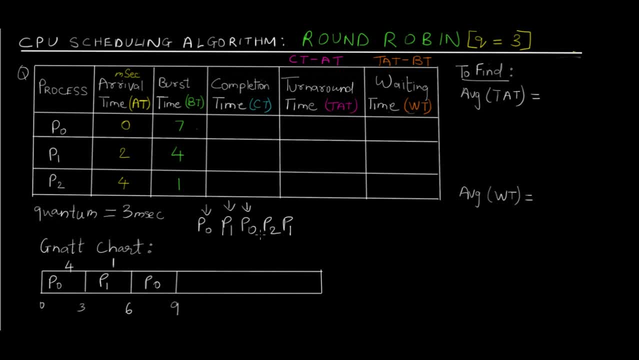 is from 6 to 9 and it will check inside the queue whether any other process is there. We know that P2 and P1 are still waiting, So P0 will again be paused at 9th millisecond. So from 6 to 9 it processed for 3 milliseconds and it required 4 milliseconds. So we still 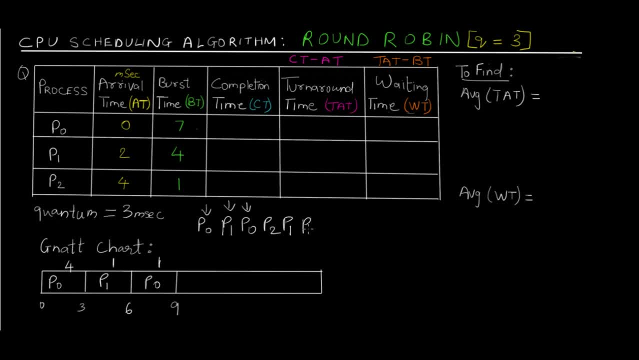 have 1 millisecond, which is needed by P0. Then we just need to add it again inside the queue. Now CPU will move to P2.. Now P2 is being processed for the first time, but we know that P2 requires only 1 millisecond. 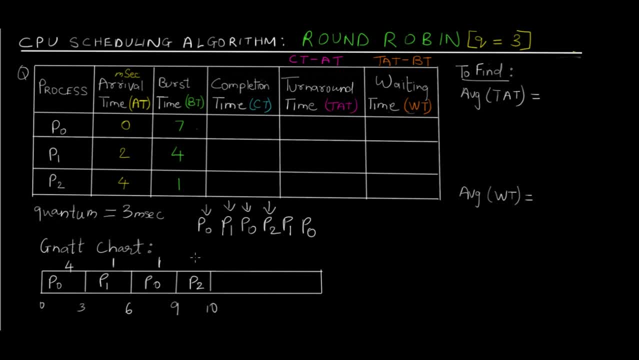 So from 9 to 10, CPU will process P2 and it will completely finish it. So writing 0 over here, which means that P0 is, or which means that P2 is completely processed. So now it will move to P1.. Now we don't need to add P2 over here, because P2 is completely finished. 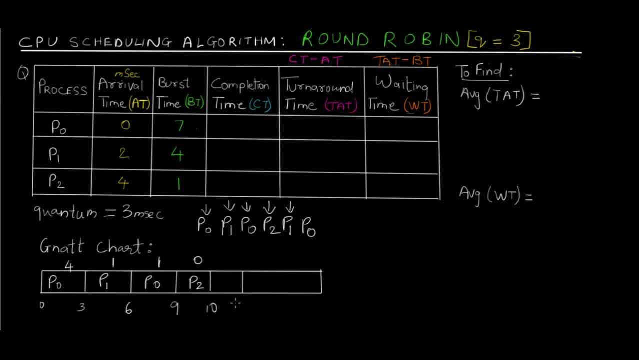 by the CPU. Now P1 requires 1 millisecond. So from 10 to 11, P1 will be processed and you can cancel this out. and you can cancel this out as well. You can write down 0 over here, Because P1 is also finished over here, and then it will move to P0.. Now P0 is the last. 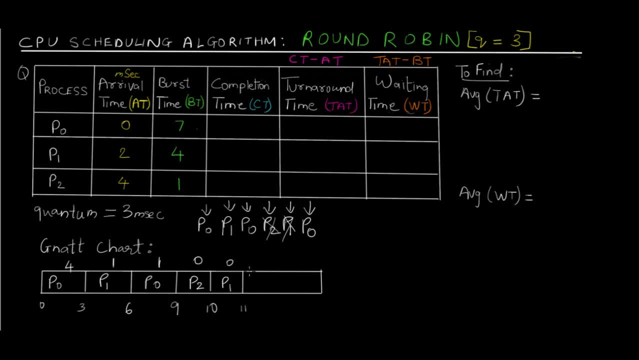 process remaining inside the queue, and you can see that P0 requires only 1 millisecond. So from 11 to 12, P0 will be executed by CPU and then it will be finished. So you can see that P2, P1, P0 have all been finished by checking the 000 number, which means that they 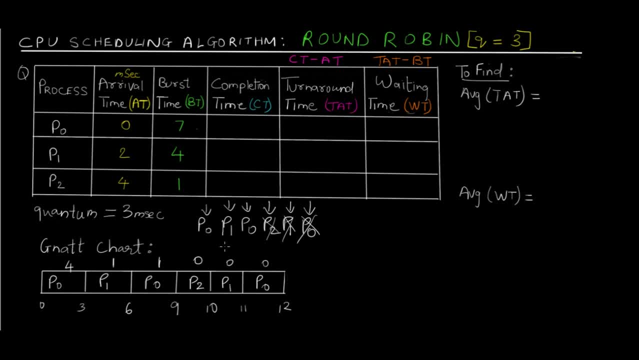 have been completely processed by the CPU. So this is the final Gantt chart. So now we can go ahead and calculate completion time, turnaround time and waiting time For P0, you can see that P0 finished itself at 12 milliseconds, So you can just write down 12. 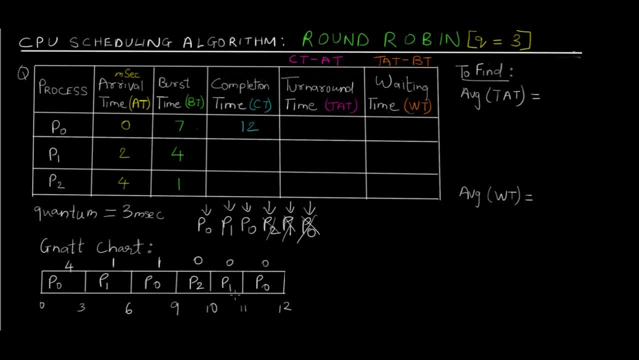 over here. For P1, you can see that the last instance of P1 inside this Gantt chart is this and it got finished at 11 milliseconds. and for P2, you can see that it was finished at 10 milliseconds, so just write down 10 over here. Now we have turnaround time, which is 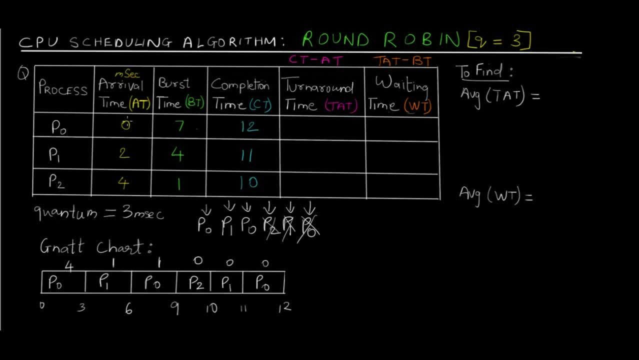 given by the formula completion time minus arrival time, So 12 minus 0, which is 12.. We have 11 minus 2, which is 9, and 10 minus 4, which is 6.. Now the waiting time is turnaround time minus BERT time. So turn around length minus BERT time. so turn around length minus. 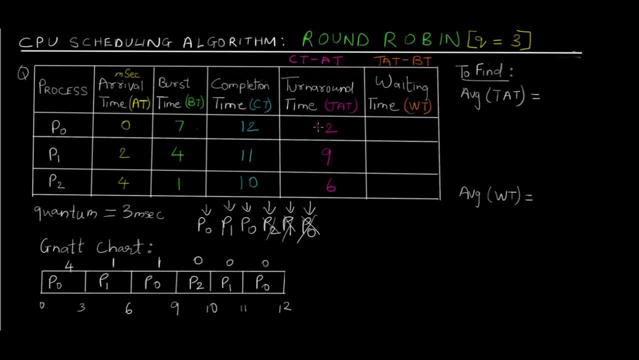 time, so turnaround time is 12 and arrival time or the burst time here is 7. so 12-7 will give us 5, 9-4 will give us 5 and 6-1 would give us again 5. so each of the process had. 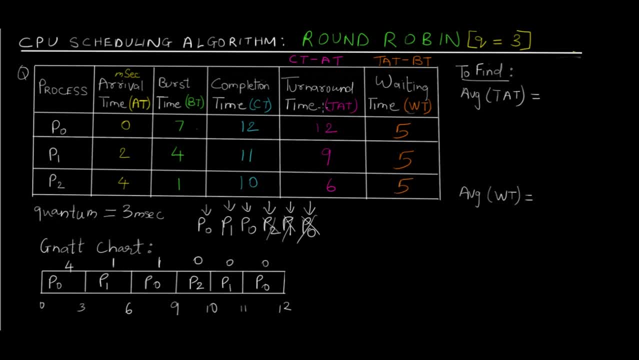 to wait for 5 seconds. now, if you don't know these formulas, you can still find out turnaround time and waiting time by knowing what they actually mean. so turnaround time is the time spent by the process inside the queue. so for p0, we know that it came in at 0th second and 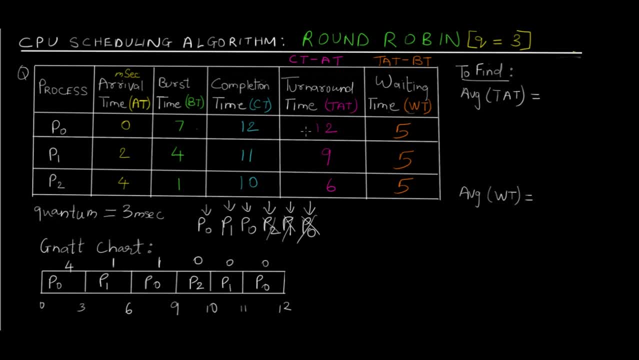 it completed at 12 seconds, so it spent total 12 milliseconds inside the queue. so that is the reason why the turnaround time is 12. similarly, you can calculate that for p1 and p2 and the waiting time is the time it had to wait. so you can see that p0 came in at 0th second.